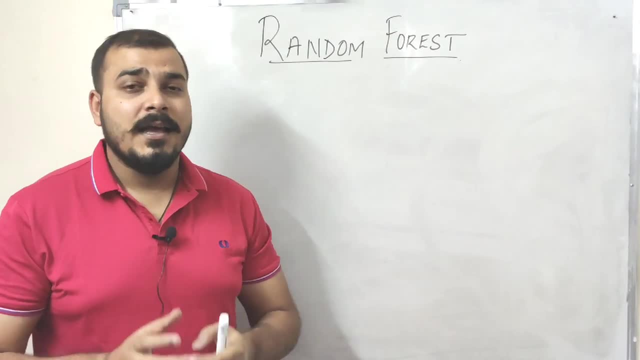 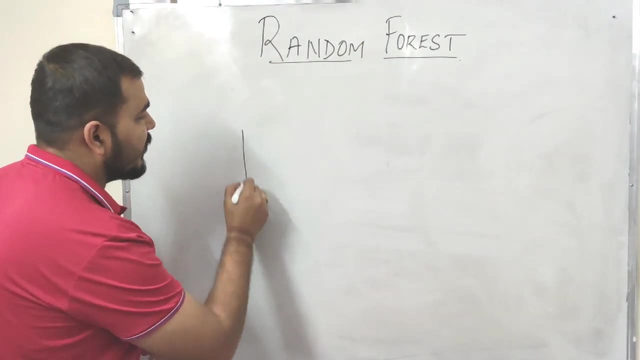 So random forest classify or a regressor is basically a bagging technique and we are going to discuss both of them in this particular session. So let me just consider and let me just show you some examples. Suppose I have a data set. Now how does random forest basically work? 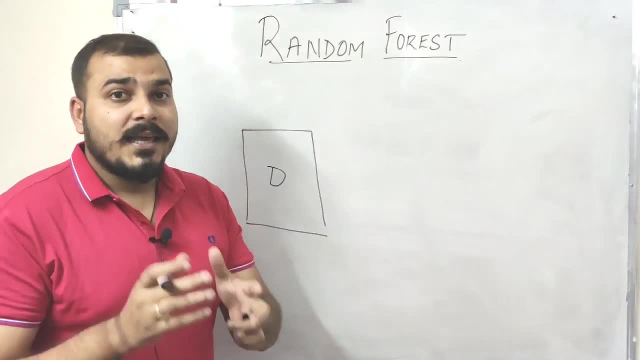 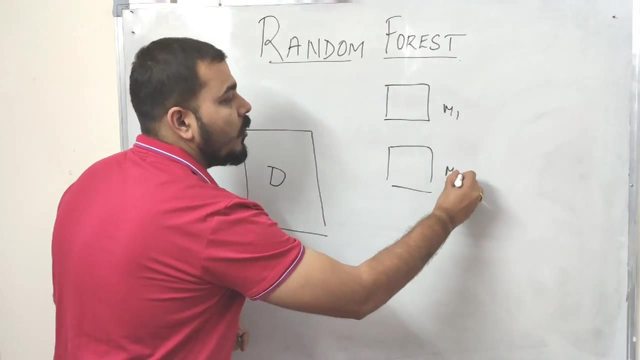 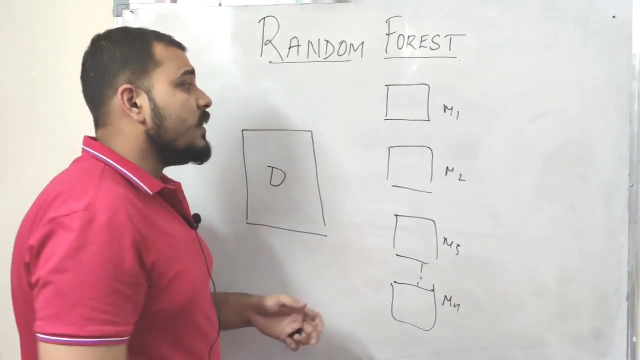 Suppose this is my data set D. Now I told you that in bagging we basically have many base learners, base learner models. So this: suppose this is my M1 model, This is my M2 model, This is my M3 model and many more models like this. Okay, so suppose this is my MN model. Now when? 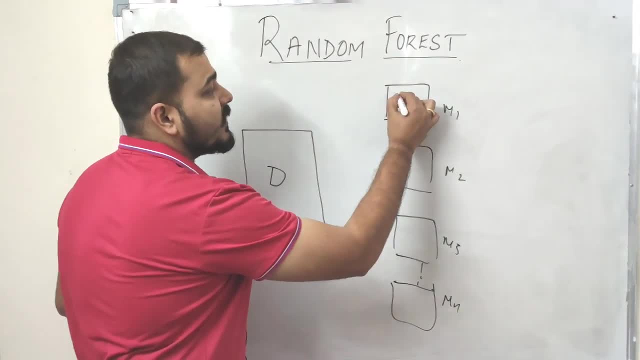 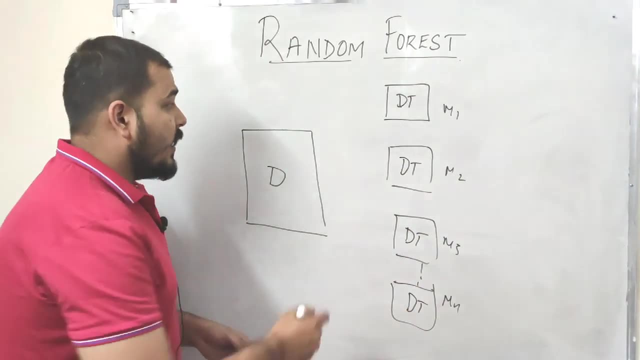 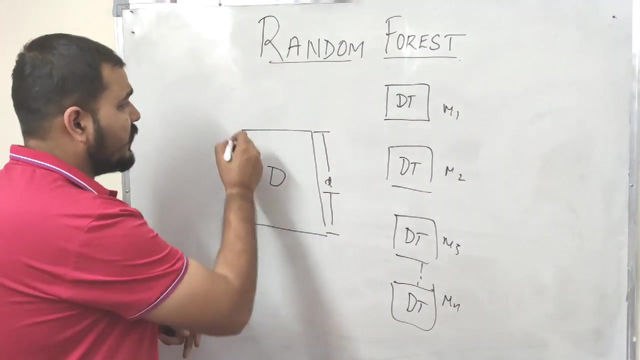 we are designing this particular model in random forest. this model is basically called as decision trees. We are going to use decision trees in this model and, as I had explained in the bagging technique, suppose in this particular data set we have D records- Okay, D number of records and M number of columns. Suppose I have that. 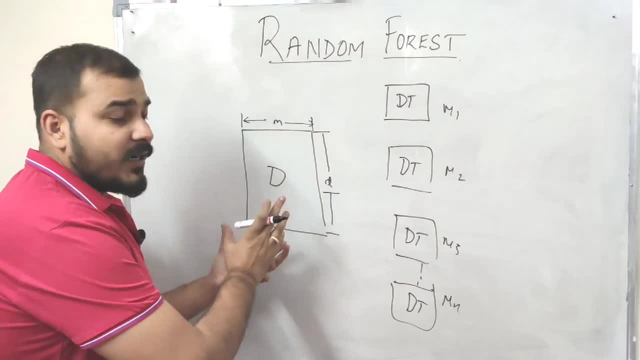 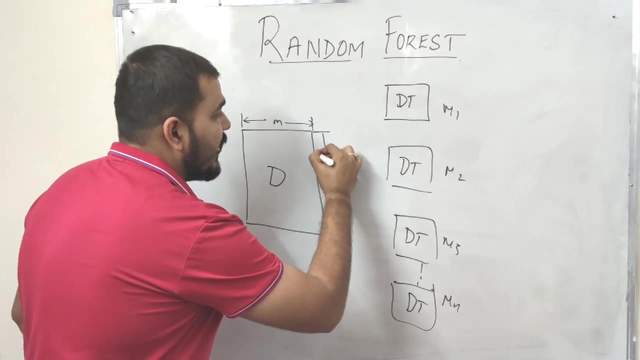 many columns: M number of columns. So what we do is that from this particular data set, we will be picking up some sample of rows and some sample of features. Okay, so, initially I'll pick up some sample of rows. I'll say it as row sampling. row sampling with replacement. 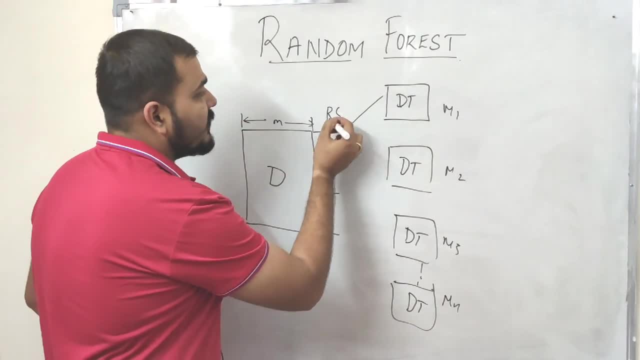 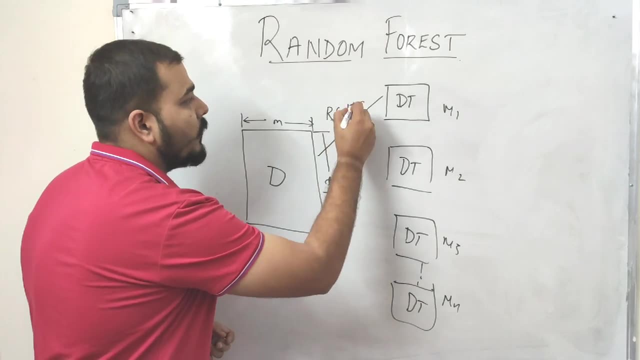 I'll just tell you what is that particular replacement term means. So I'm going to take rows from this particular data set And, similarly, I'm going to pick up some columns. Okay, or I can also write this as feature sample. So FS, okay, feature sample replacement. Now that is how. 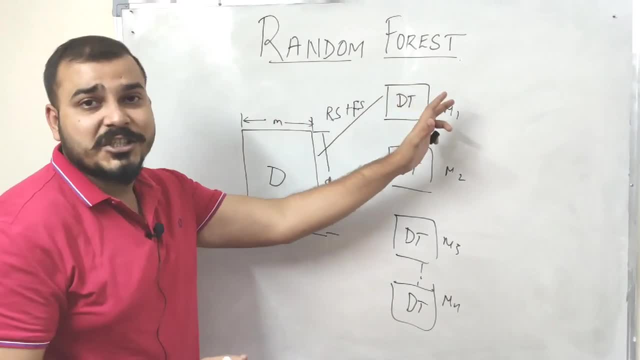 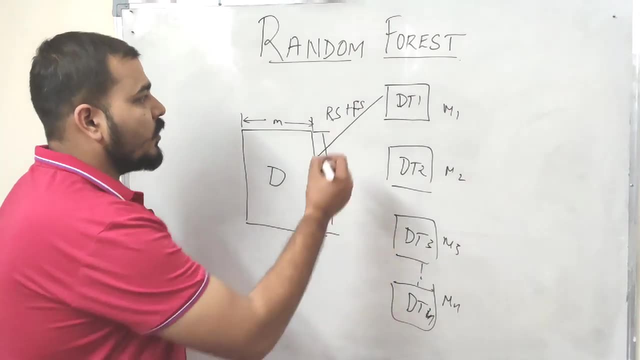 bagging words works right. We will be taking some amount of rows, giving to our decision tree one. So this is really my decision tree one. decision tree two, three, four, N, Okay, so all this decision tree. Suppose I say that this particular data set is basically D dash Always remember. 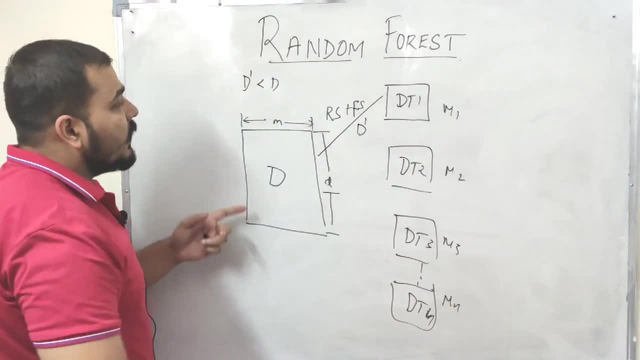 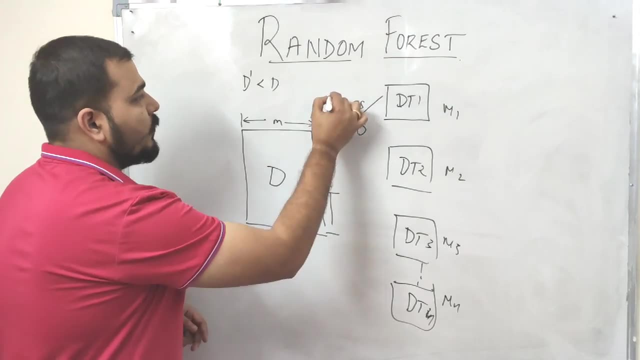 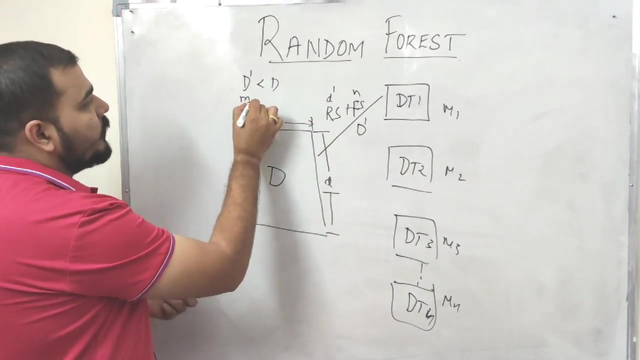 when I say D dash, D dash is always less than D because the number of records from here. I'm just taking a sample of records And suppose, if I consider that I have taken N suppose small D dash rows and N columns right N number of features. So always remember this M. 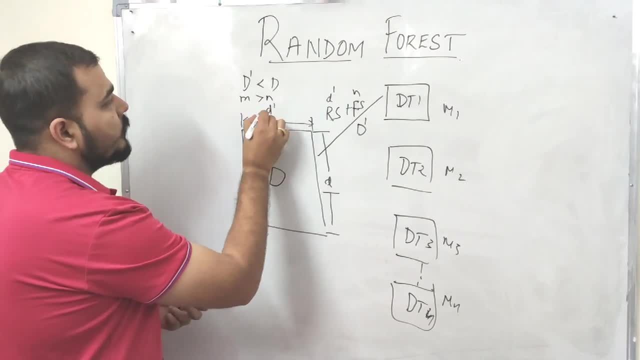 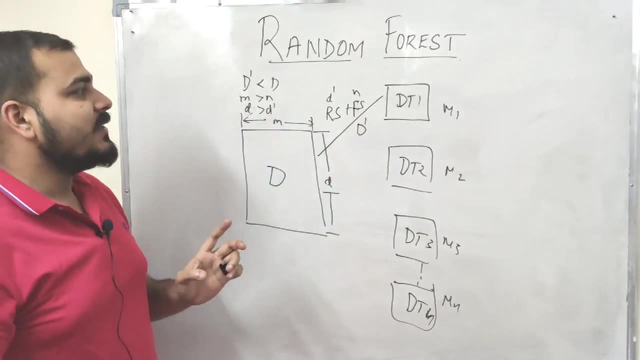 will always be greater than N and this D dash, this capital D, will always be greater than D dash or small D. I'll say it as small D because the total number of records I've written as D. Okay, so always remember that, guys. I am going to take some. 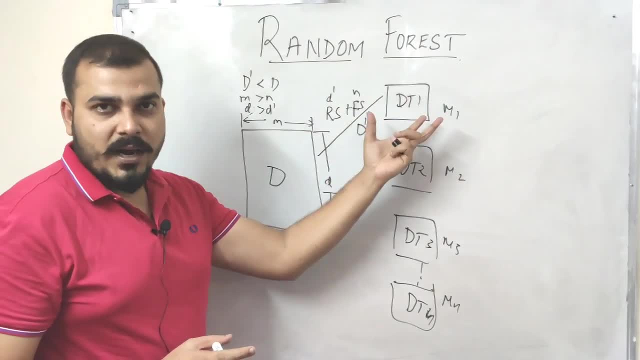 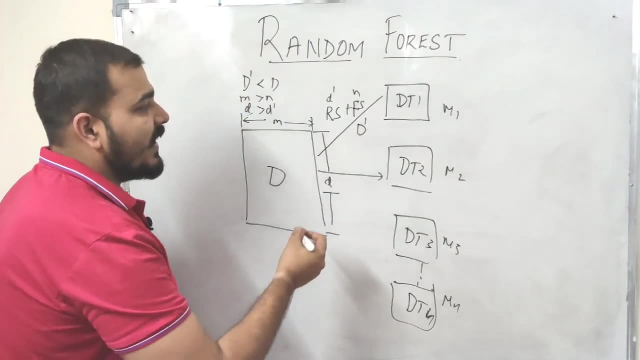 number of rows. some number of features give it to my decision tree one. This decision tree one will get trained on this particular data set. Now, similarly, for my decision tree two. what I'll do is that, again, this row sampling will happen with. 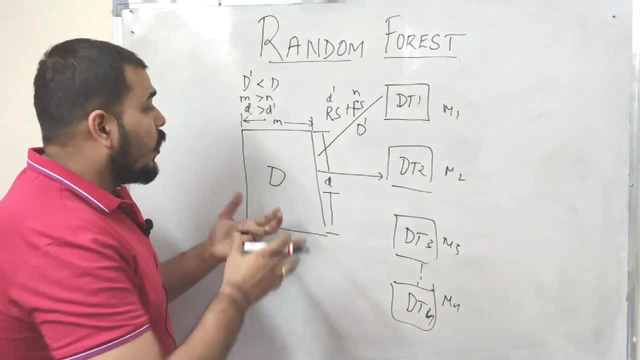 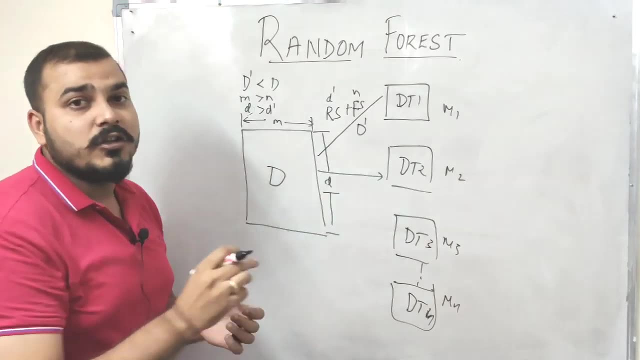 replacement. Now, what does with replacement mean? is that over here, suppose from this particular record, I have some of the records, some of the records. it may come into this particular scenario Also, when I'm doing row sampling with replacement- not all the 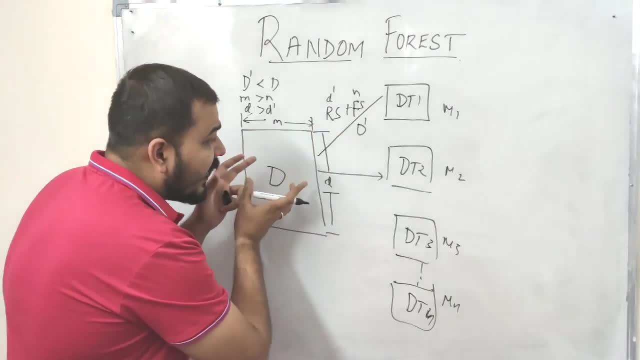 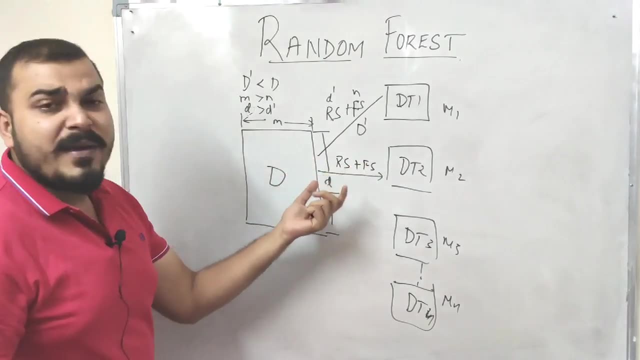 records will get repeated, But instead I'll be taking another sample of records and give to our decision tree two. So when I'm doing again a row sampling plus feature sampling over here it may be it may happen that some of the records may get repeated here, some of the features may get. 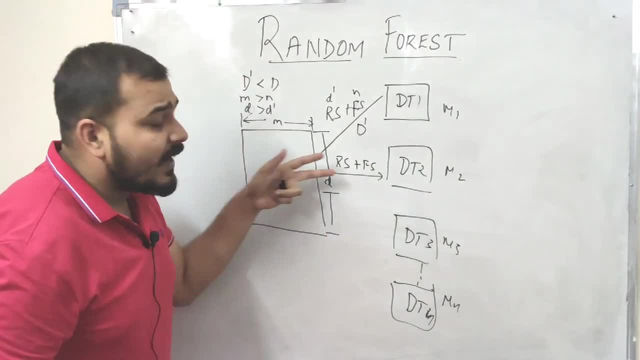 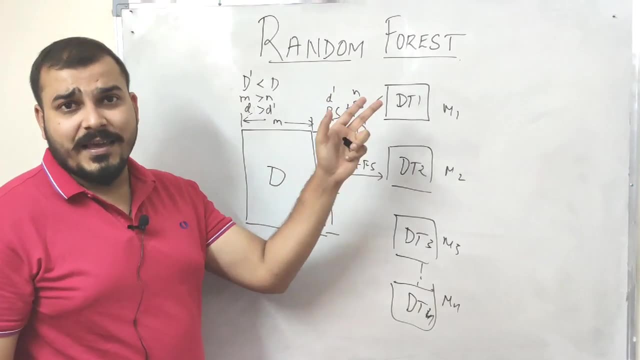 repeated here, But we are at least changing many records. Again we are doing this row sampling. okay, row sampling and feature sampling. So suppose in this particular case I had given feature 12345.. Suppose in this particular case I'll give other features, like feature 134567, like 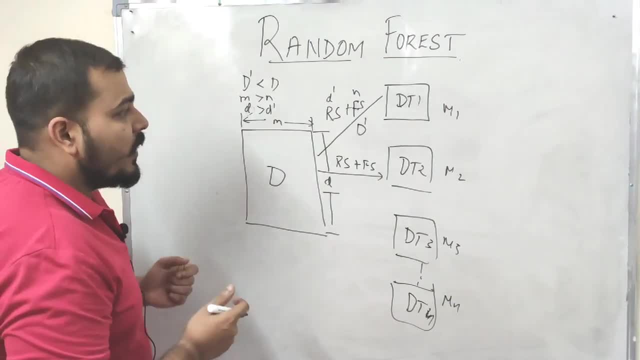 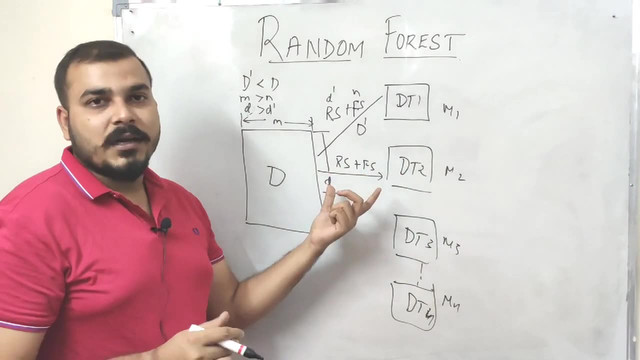 that And, similarly, that row sampling also happens in the similar way. Now, after doing this row sampling and feature sampling, I'll give this particular records to my decision tree, to this will get trained on this particular data. Similarly for every decision tree, this thing is going to. 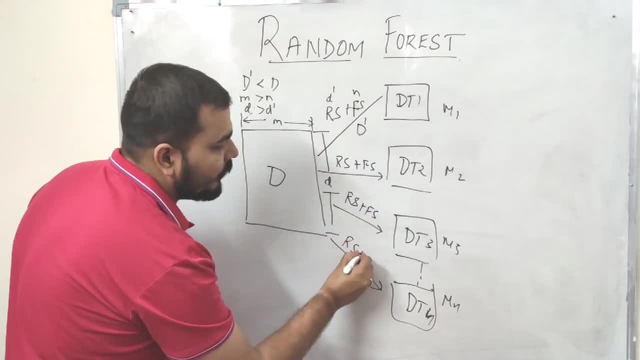 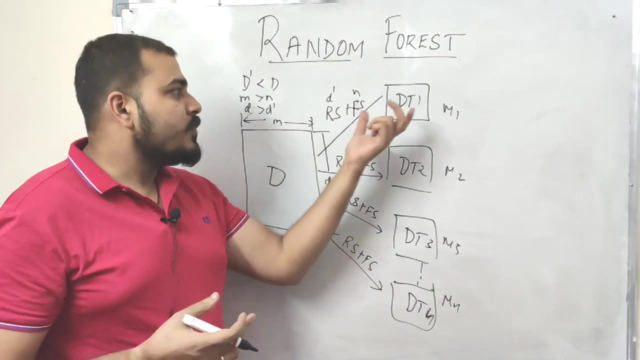 happen where you're going to perform row sampling and feature sampling. Okay, row sampling and feature sampling. Now this decision tree gets trained on this particular data. okay, and now it will be able to give the accuracy, or it will be able to give the prediction. Now the next. 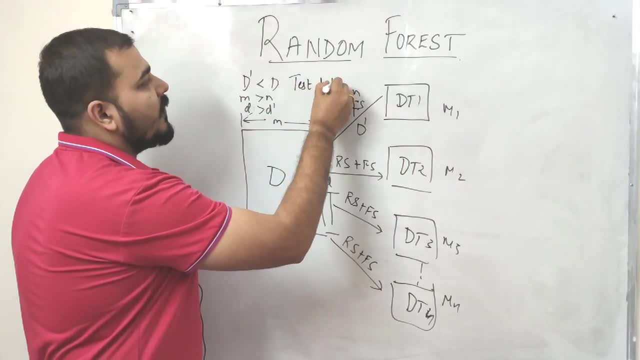 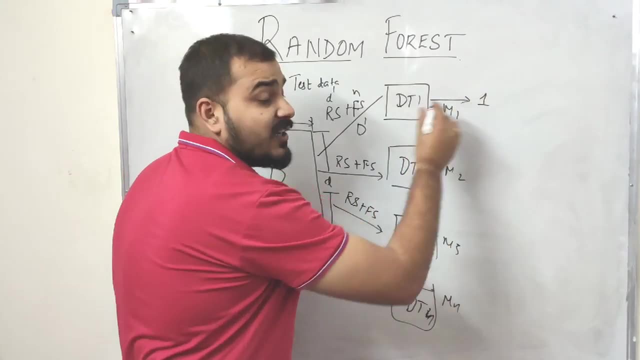 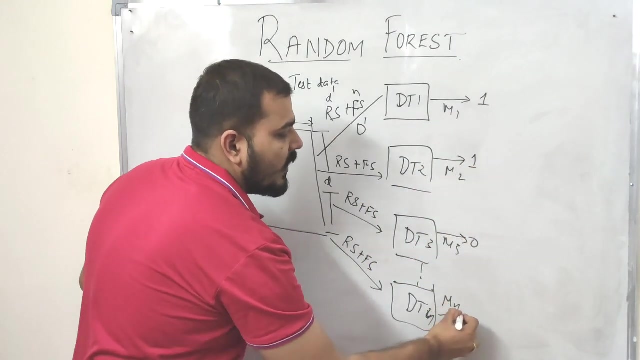 thing is that whenever I get my test data, whenever I get my test data, suppose I'm giving one record of the test data into this particular decision tree. one suppose decision tree. one suppose I'm considering a binary classification problem decision tree: one gives me one, this also gives me one, this gives me zero. and suppose this gives me one. 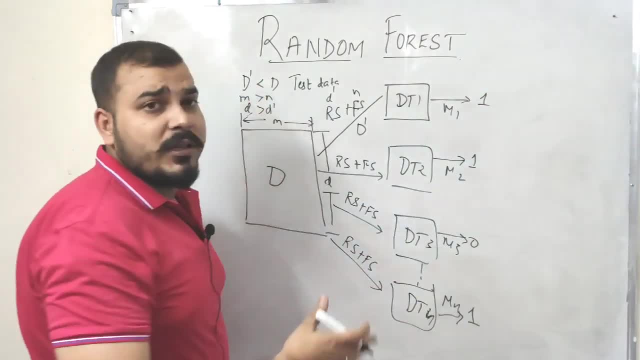 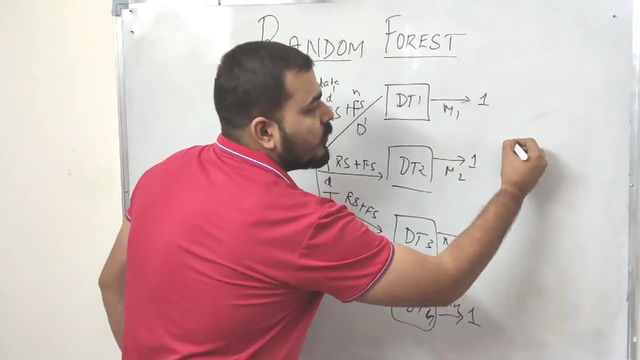 okay, Now, when we see over here, finally, we know that this is my bootstrap. And now, according to the bagging, finally, after aggregate it right. So for aggregating I'm going to use the majority of the data. 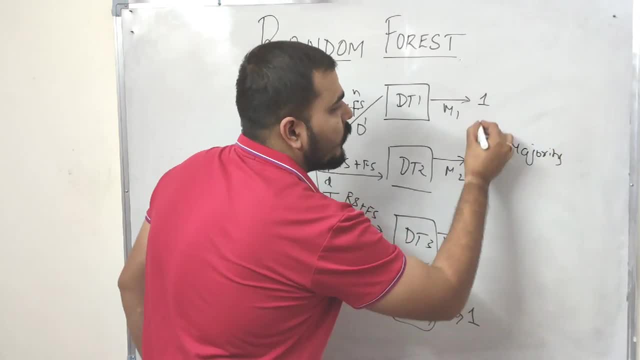 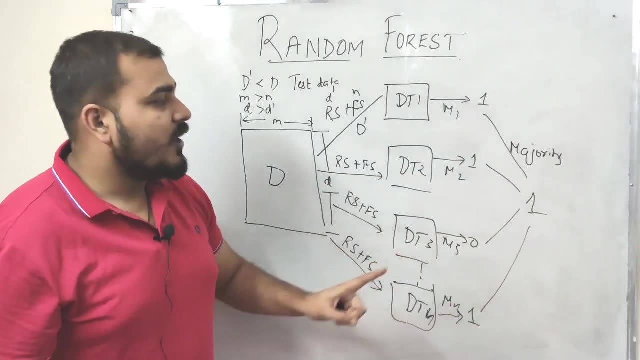 So for aggregating, I'm going to use the majority of the data. Now, when I use the majority vote, I know that the maximum number of models that are basically saying the output is like one. So I can see one, two, three models is basically saying it as one. So, finally, my output is basically one. 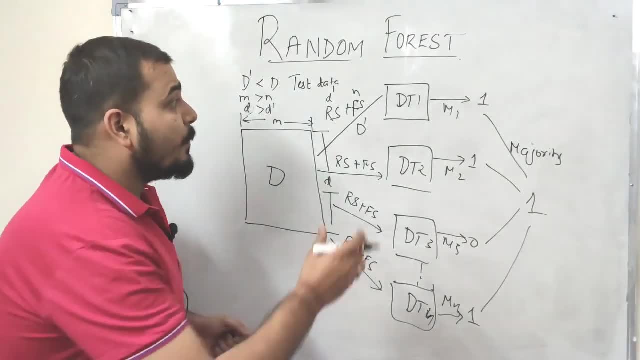 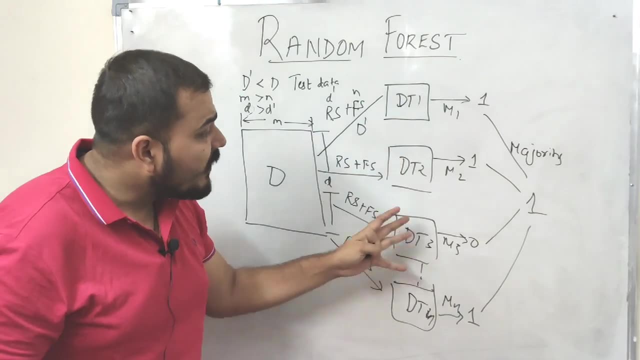 Now this is how a decision random forest basically works. The base learner is decision tree. Now you need to understand one more thing in this. What is happening when we are using many decision trees in this particular random forest? Guys, you should know that. 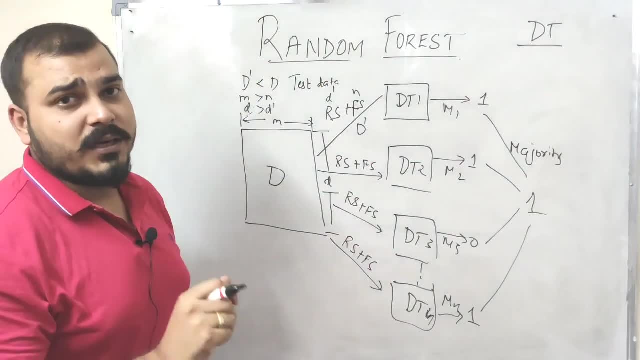 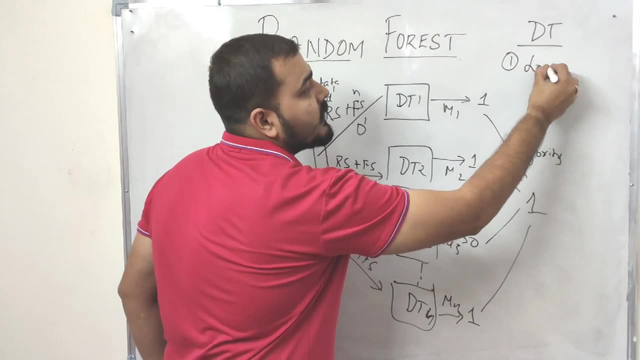 You should know that. You should know that Decision tree: whenever I use decision tree, it has two properties. Suppose if I'm creating a decision tree to its complete depth, So when I do that, it basically has low bias and high variance. 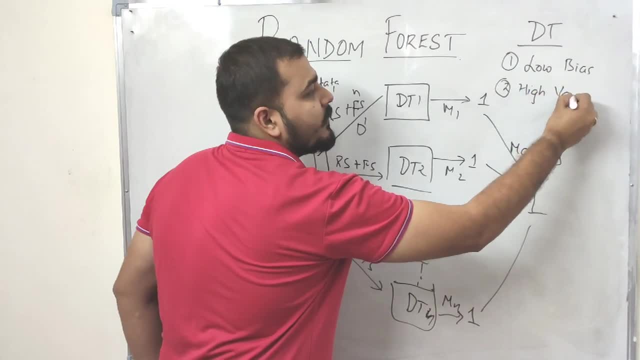 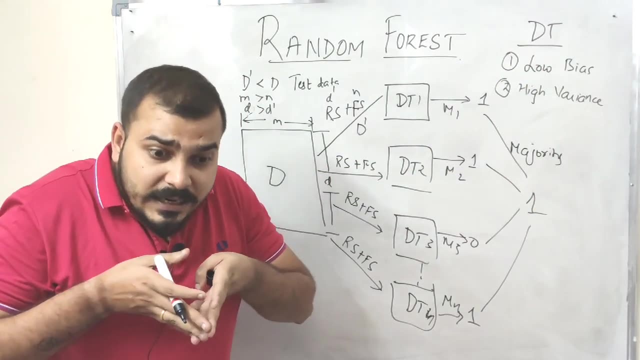 I'm going to explain about what is low bias and high variance. Just let me write it down first of all. So low bias basically says that if I'm creating my decision tree to its complete depth, then what will happen is that it will get properly trained for our training data set. 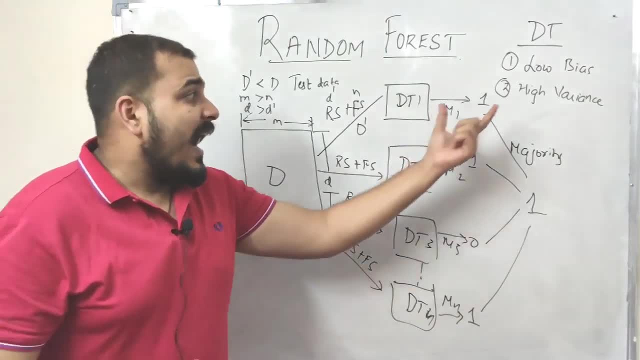 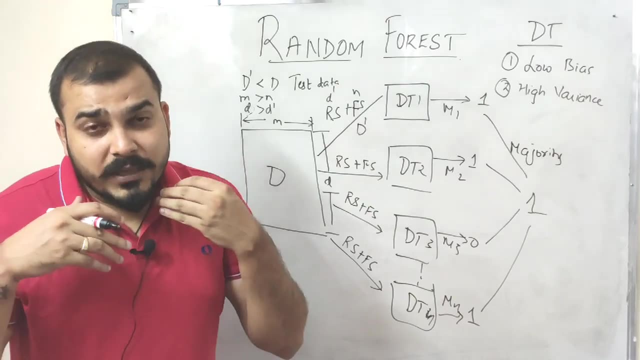 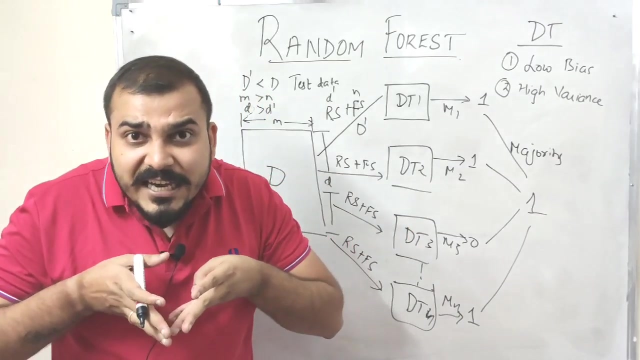 So the training error will be very, very less. High variance basically says that now, whenever we get our new test data, those decision tree, they are prone to give larger amount of error, So that is basically called as high variance. So, in short, whenever we are creating the decision tree to its complete depth, 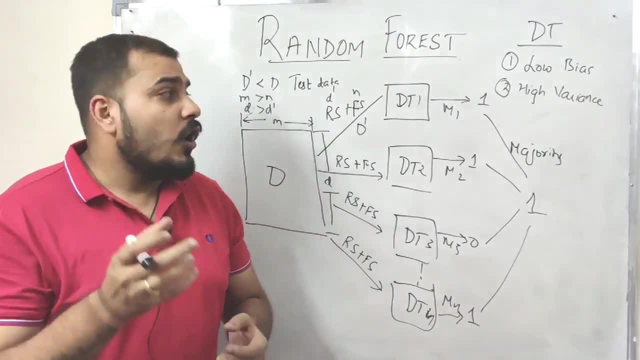 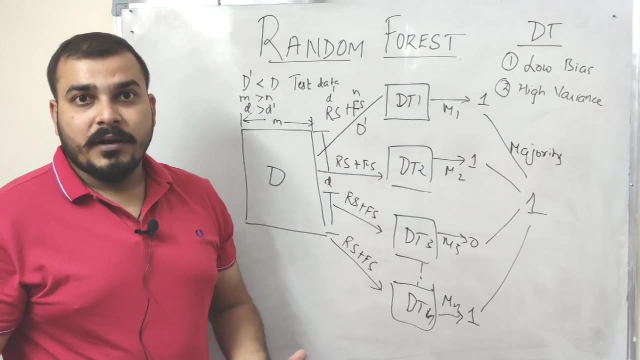 it leads to something called as overfitting. So now, what is happening in random forest? In random forest, I am basically using multiple decisions. I am using multiple decision tree, right, And we know that each and every decision tree will be having high variance, right. 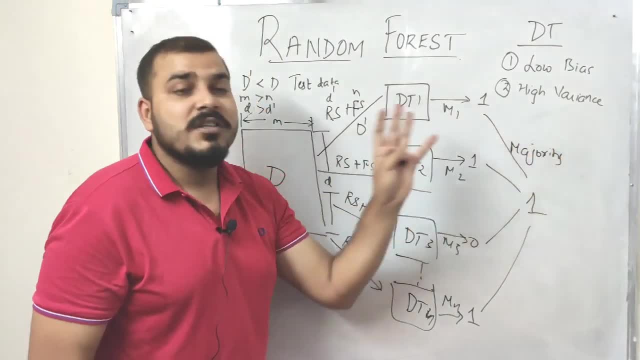 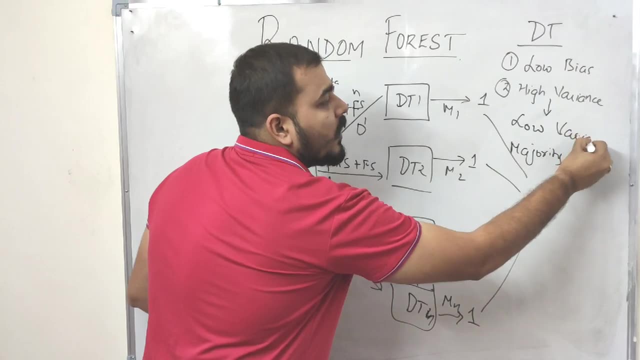 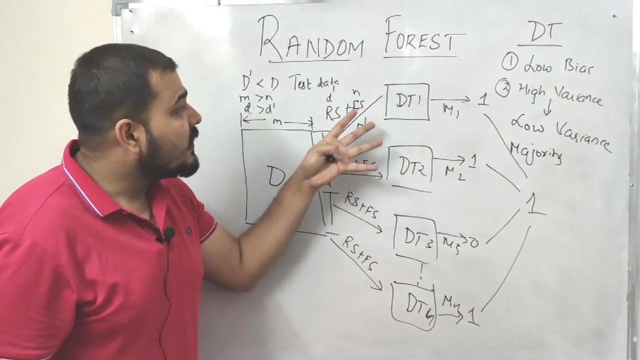 But when we combine all the decision tree with respect to this majority vote, what will happen is that this high variance will get converted into low variance, Because now, when we are using row sampling and feature sampling and giving the records to the decision tree, the decision tree tends to become an expert with respect to this specific rows. 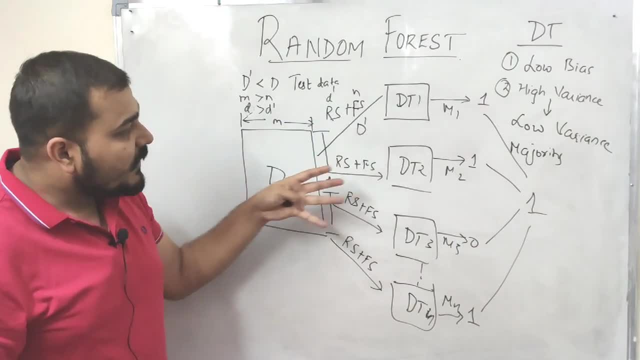 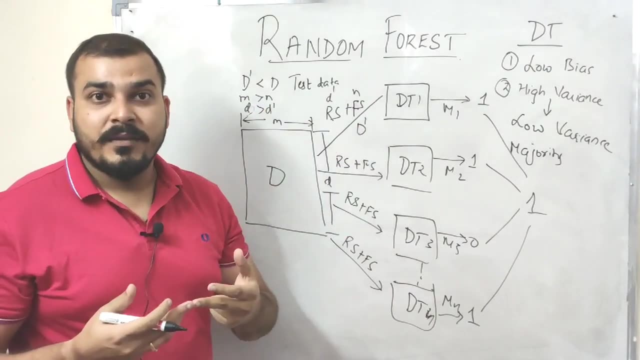 or the data set that they have. Okay, since we are giving different, different records to each and every decision tree, they become an expert with respect to those records. They get trained on that particular data specifically And in order to convert this high variance to low variance. 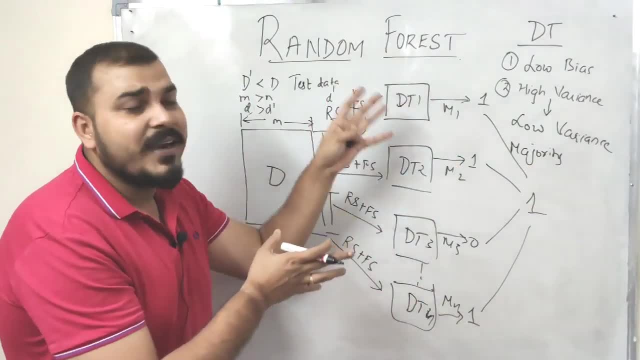 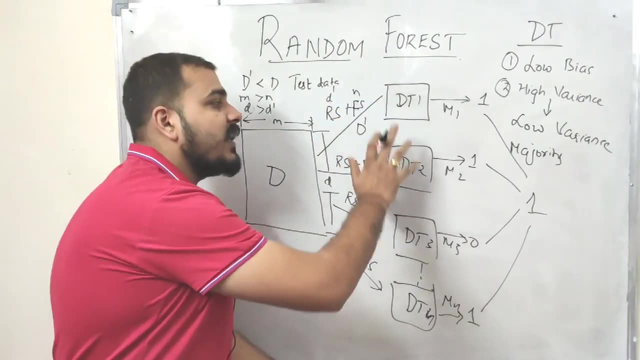 we are basically taking the majority vote. Okay, we are not just dependent on one decision tree output. So because of that, this high variance will get converted into low variance when we are combining multiple decision tree. Now one more advantage you need to understand. 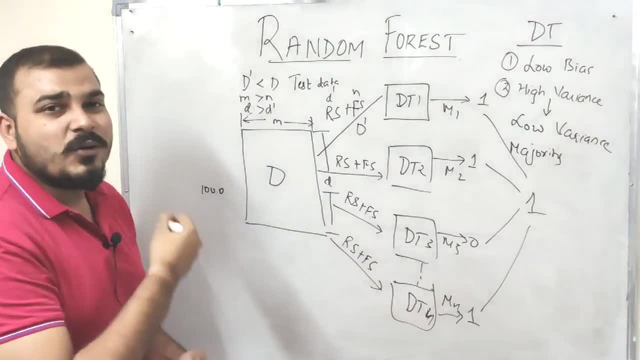 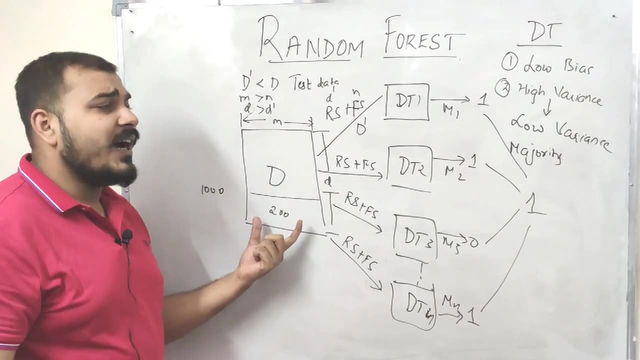 Suppose I have thousand records over here Now in this thousand records, okay, suppose I just change. let me just change 200 records. Will this change of the data impact this random forest? Now understand guys, we are doing random sampling. 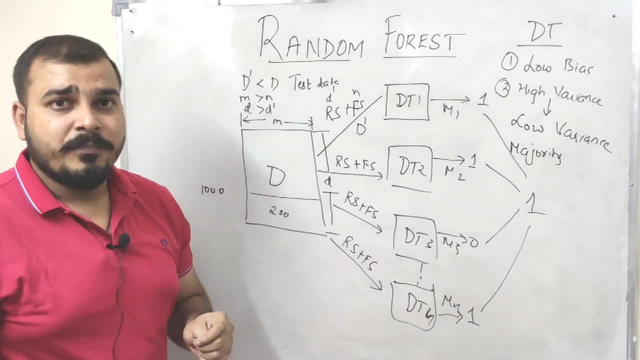 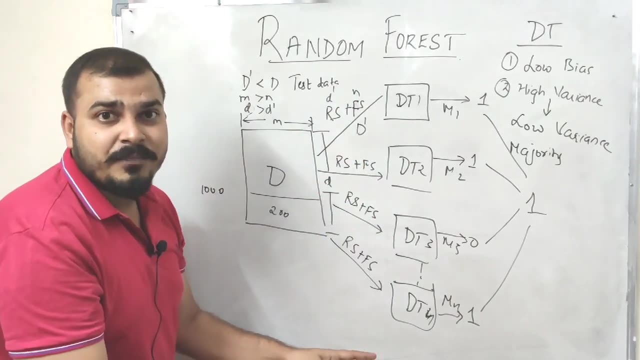 sorry, row sampling and feature sampling for each and every decision tree. Now, if I just change 200 records now, this 200 records will be properly splitted between this data decision tree. So when it is actually splitted, then what will happen is that some of the number of rows 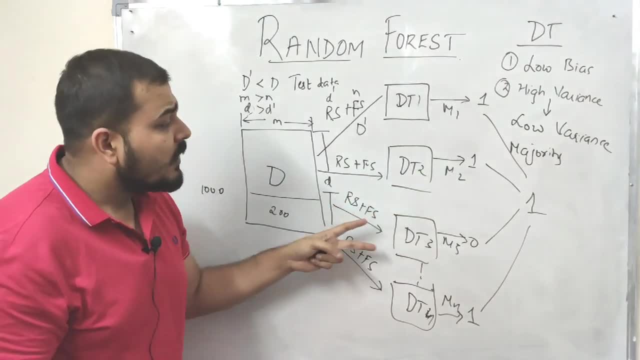 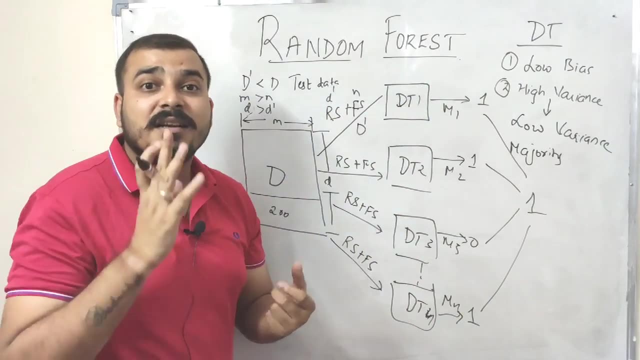 or some of the number of records will go to decision tree one, then decision tree two, then three, then four. So this data change will also not make that much impact to our decision tree with respect to the accuracy or with respect to the output. 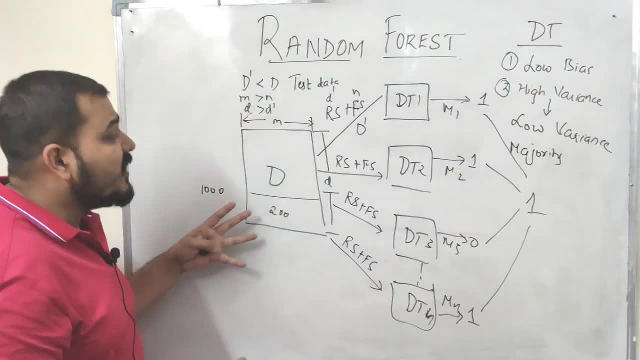 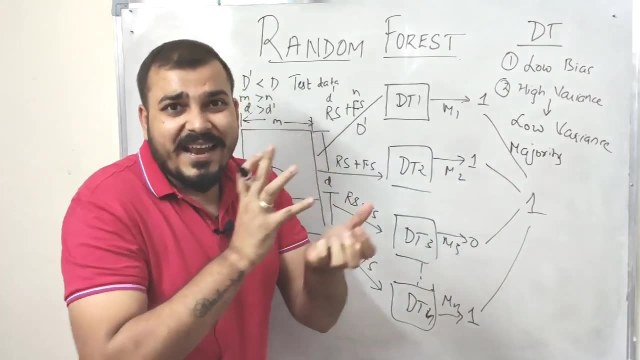 So that is why this high variance: even though whenever we change our data, whenever we change our test data, we will be getting a low variance error Or our error rate will be very, very low, Our accuracy will be very, very good. 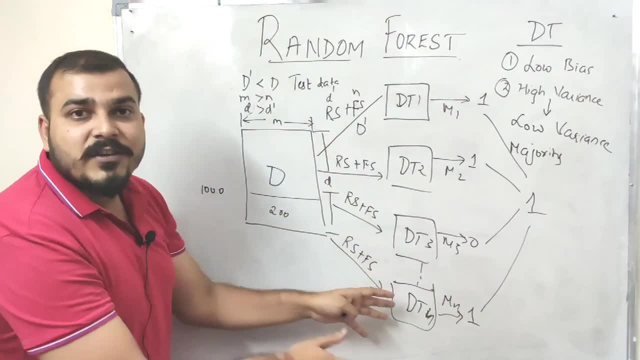 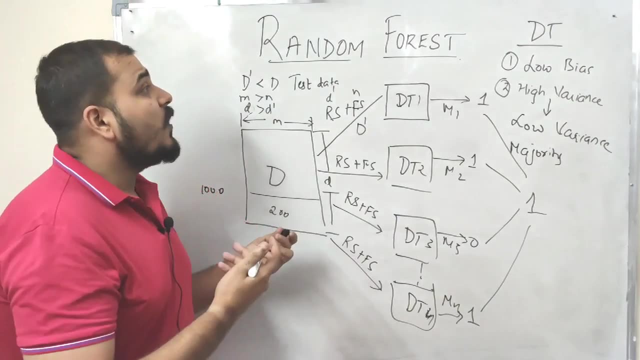 Since we are taking the majority vote, we are doing row sampling and feature sampling, giving to the decision trees. Now this is the most important property of random forest. So random forest actually works very well with respect to most of the machine learning use cases. 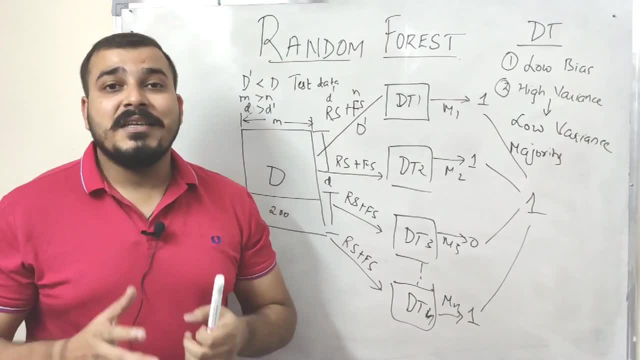 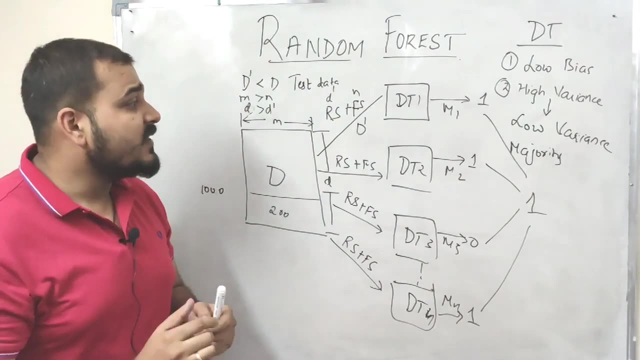 that you are basically trying to do And I've seen in most of the companies, developer have made their favorite algorithm as random forest. Let it be classifier regressor. One more point I missed out is that suppose if this is not a binary classification, it is a regression problem. 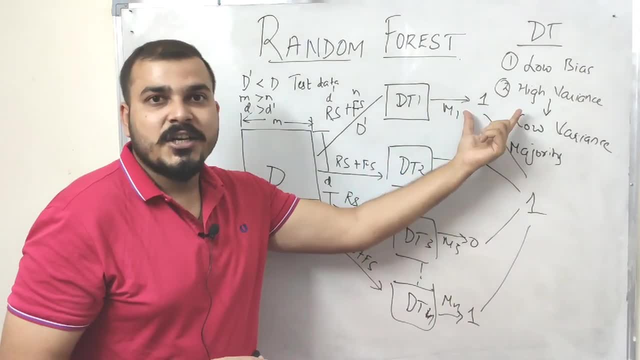 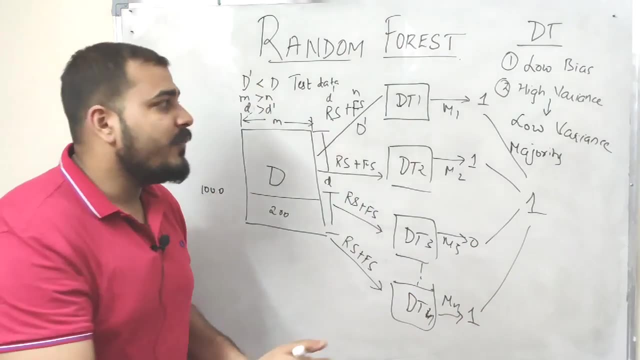 What will happen now? now, this particular decision tree, suppose it gives me a continuous value, this also gives me a continuous value. this also gives me a continuous value for that. what we do is that in regression problem, we either take the mean of all this particular output or the median of that particular output. 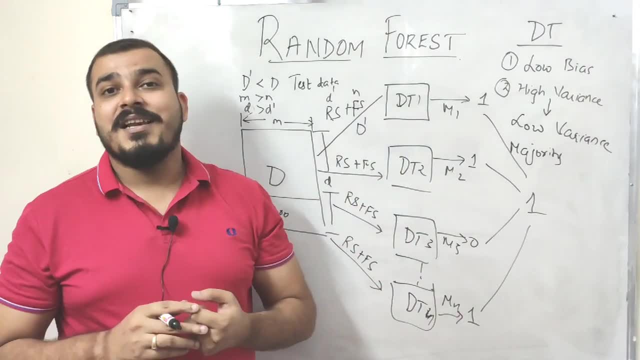 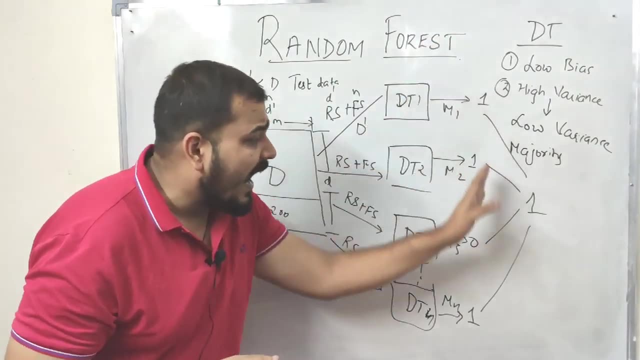 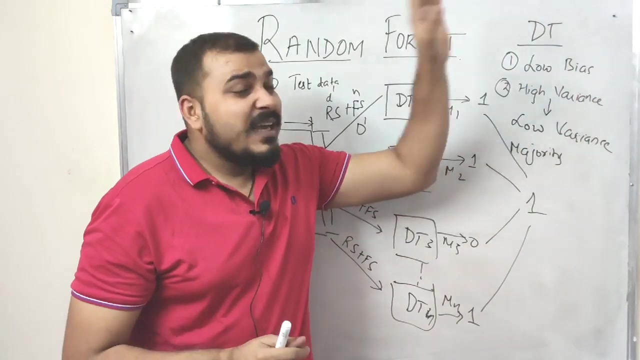 it depends on the distribution of the output, how the decision tree is basically giving. so usually the main run for is that works with respect to sklearn. it tries to find out the average of this particular output from all the decision trees and that is much as simple it. but you need to understand. if I just use single decision tree it will. 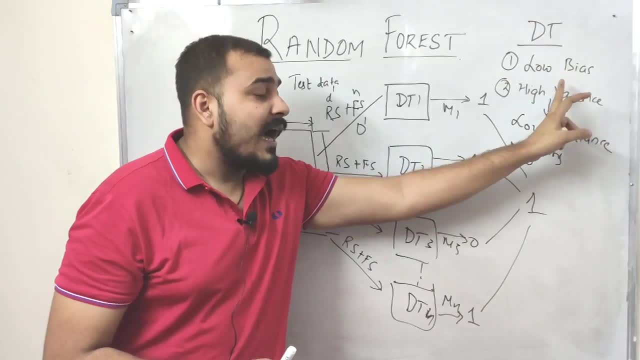 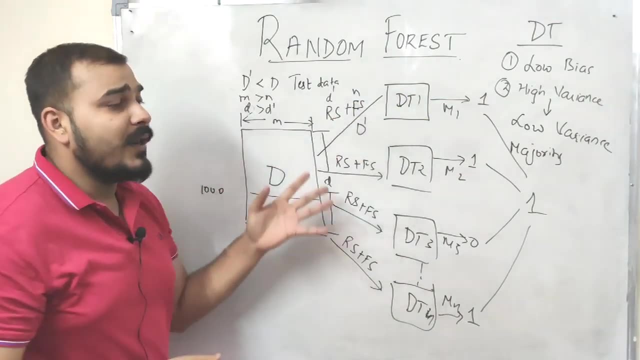 have low bias and high variance. if I want to convert this high by high variance into low variance, I have to basically use multiple decision tree. apart from that, I also have to use row sampling and feature sampling so that I will be able to convert that into low variance. that basically means our 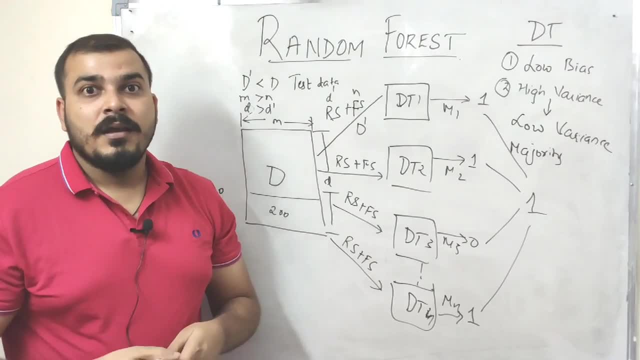 accuracy for the new data or the test data will be very, very good. so this was all about random forest and I have explained you before about random forest and I have explained you before about random forest and I have explained you both about classifier and regressor, only the difference between classify and 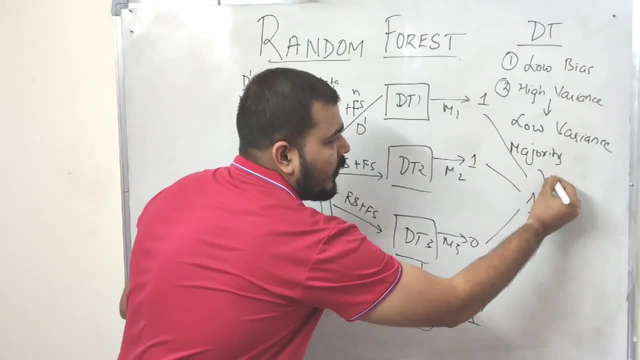 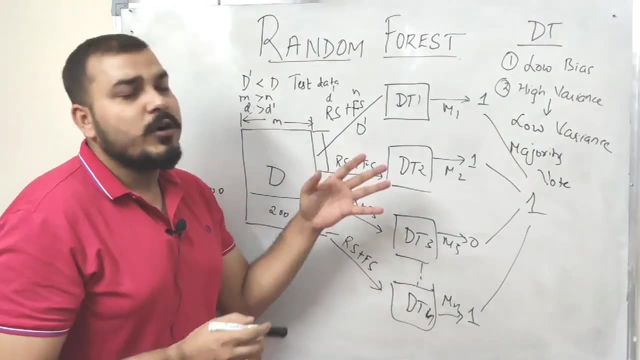 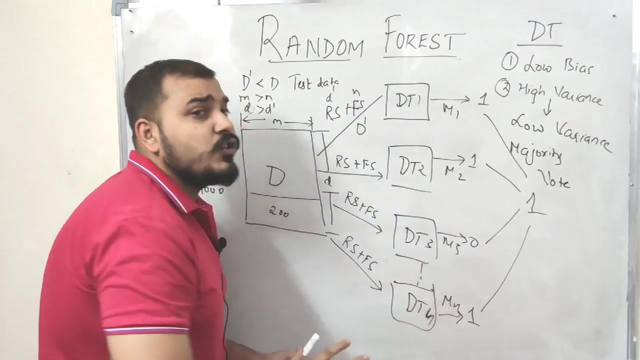 regressor is that classify uses majority vote. I'll just write it down: majority vote. whereas in the case of regression, it will actually find out the mean or the median of the particular output of all the decision trees. now, the hyper parameter that you have to basically work on in that how many decision trees? 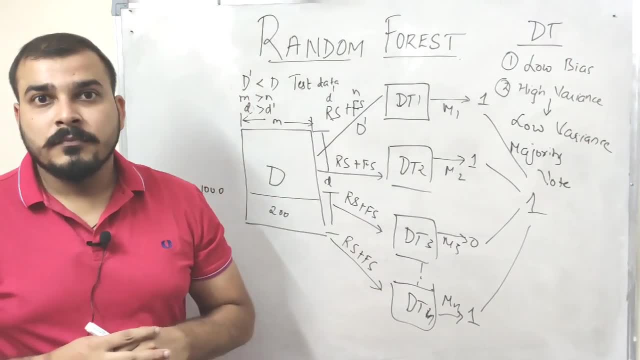 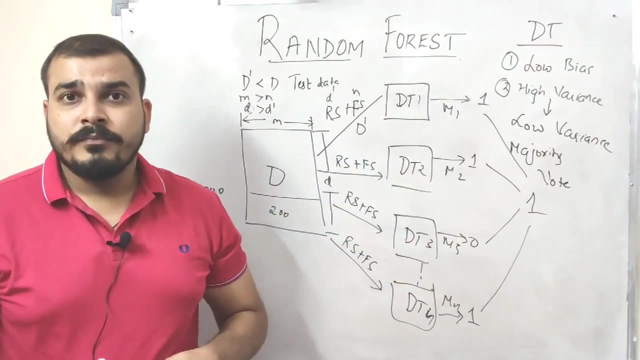 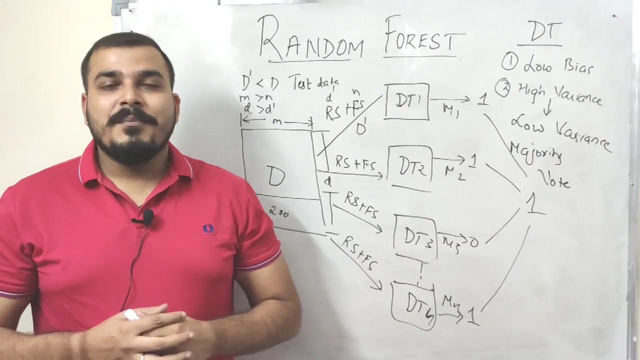 you have to actually use for the random forest, okay, how many decision trees you have to basically use. so by with the help of hyperparameter, you will be able to work that out. okay, so this was all about the video of random forest classifier and regressor. I hope you like this particular video please. 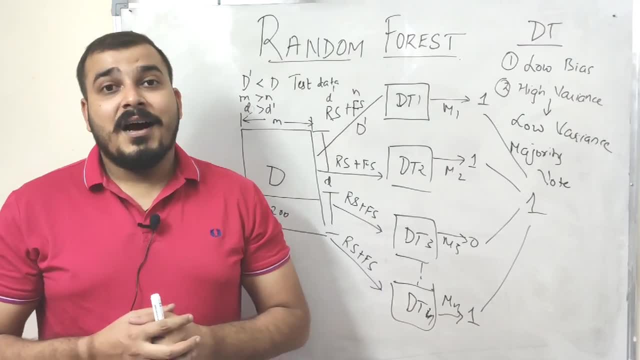 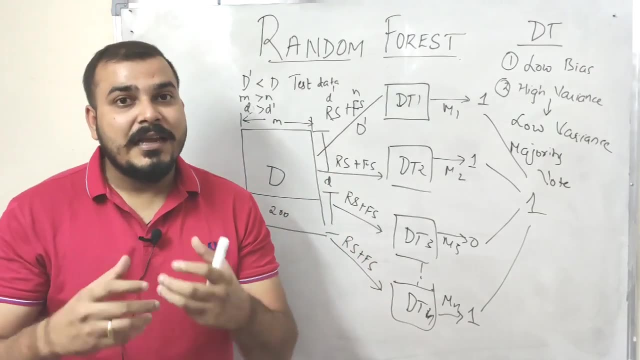 make sure you subscribe the channel. share with all your friends. please share with all your friends, whoever require this kind of help, because all the materials over here are free to share with as much as people as you can. I'll see you all in the next video. have a great day. thank you one and all. you. 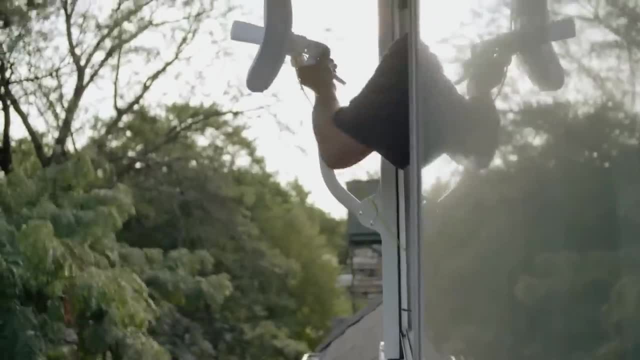 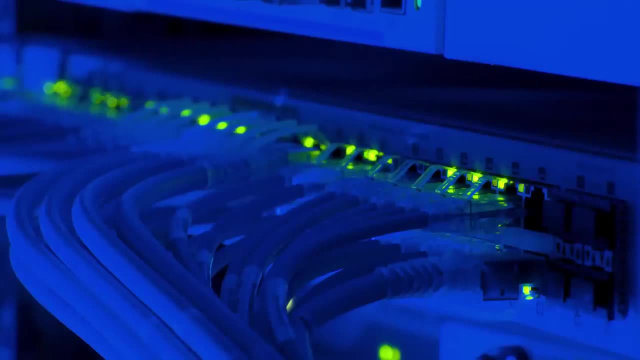 Securing your network is essential, but it isn't difficult. Even if you are not the best friends with technology, you'd be surprised how insecure your home network is and how vulnerable you are on an open Wi-Fi. If somebody gets into your home network, they could potentially collect your 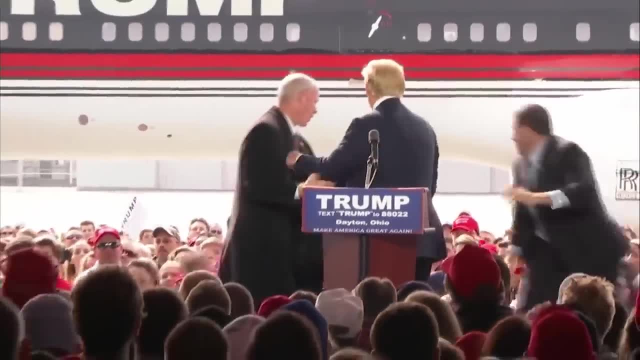 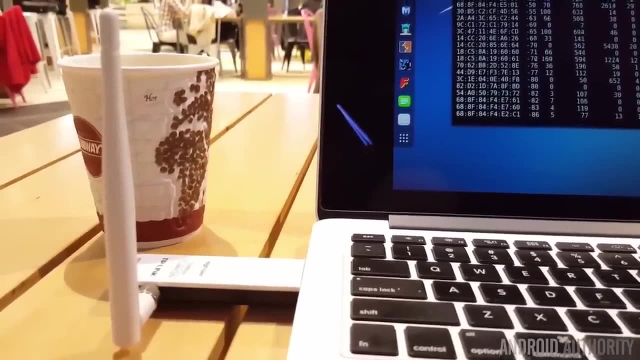 private information or send death threats to the President of the United States from your IP address. If you connect to a hostile network, your phone could be controlled by hackers forever and you wouldn't notice until you lose access to all your accounts and end up facing insane.